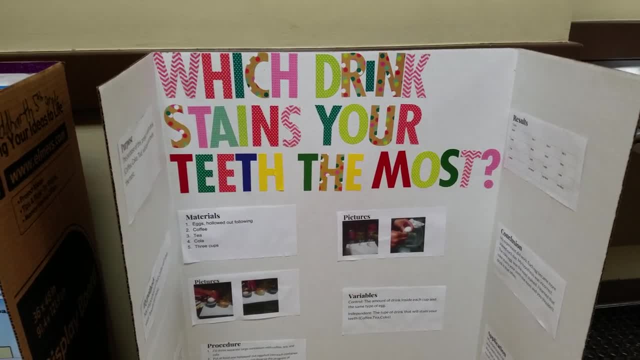 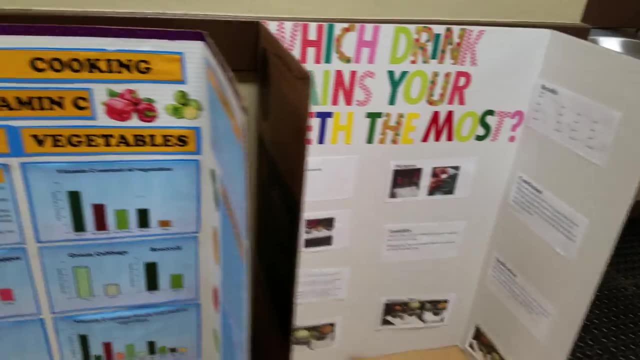 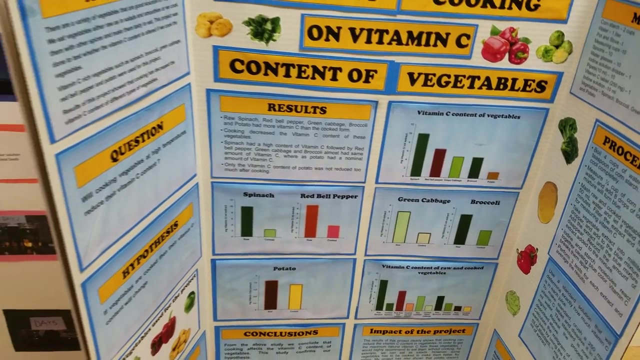 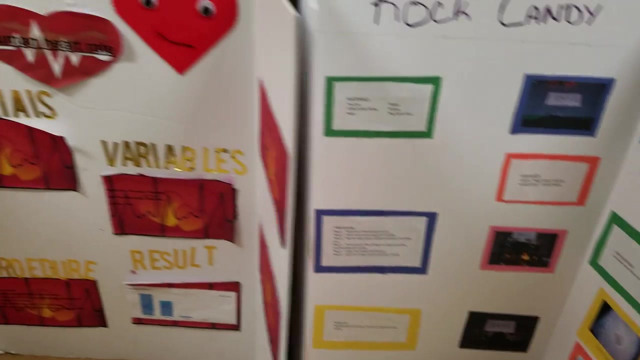 We're going to talk about science fair projects today. Today, this project is: which drink stains your teeth the most? All right, this next project is effects of cooking on vitamin C. Okay, this next project is rock candy. Here we have human heart rate. 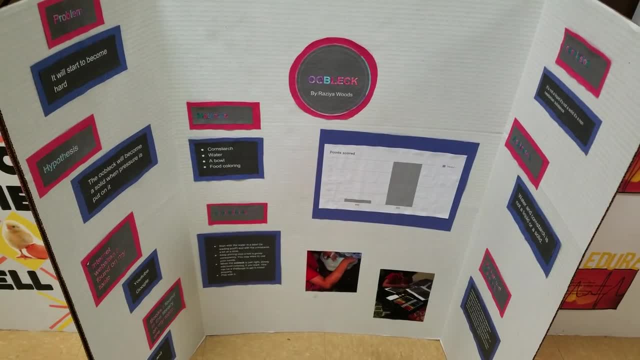 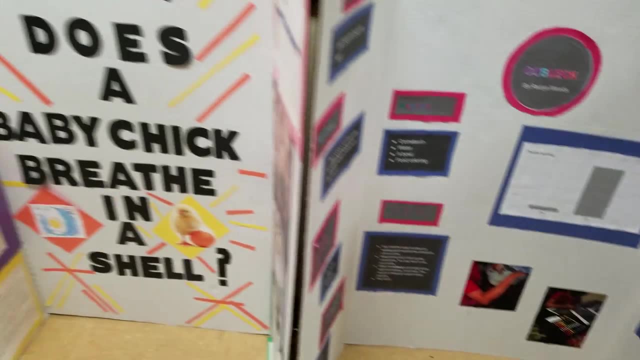 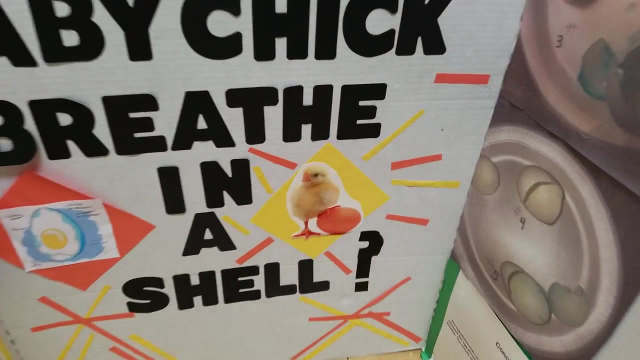 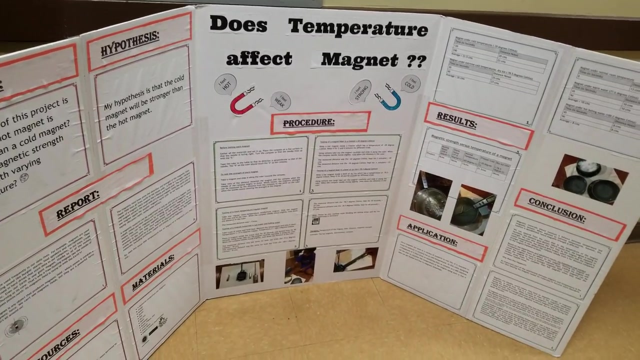 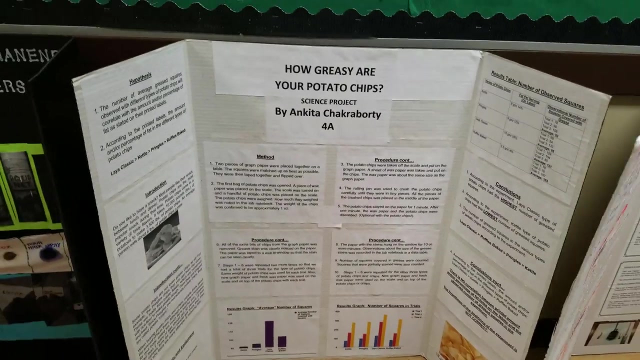 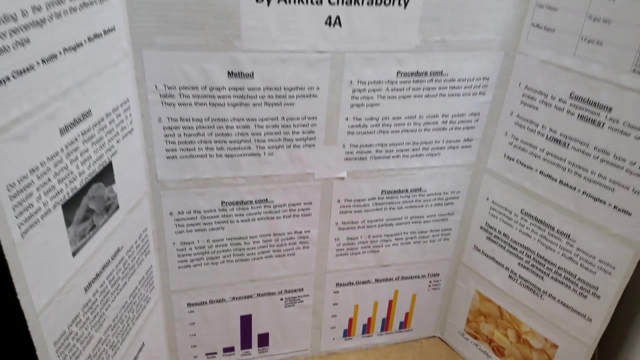 Okay, this next project looks a little interesting. All right, here we have how does a baby chick breathe in a shell Moving along, does temperature affect magnet? And here we have how greasy are your potato chips? Here we have exploring the permanence of permanent markers. 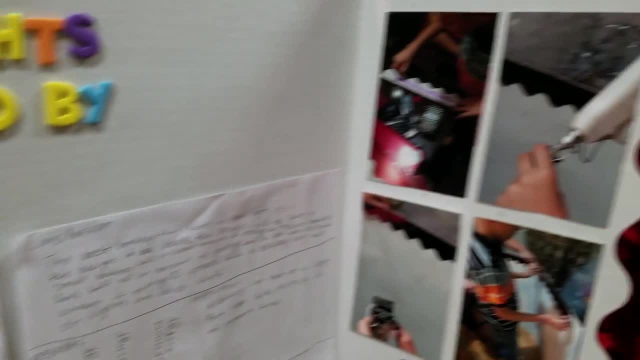 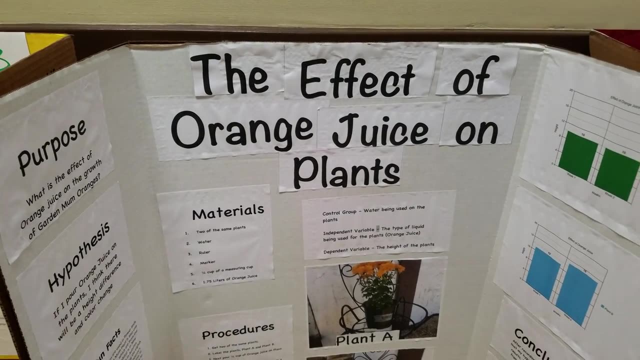 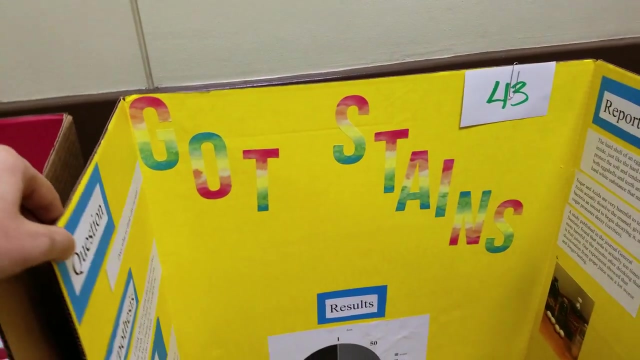 Here is LED lights operated by a battery. This project is the effect of orange juice on plants. We have nose, nose and x-rays. on the right hand side, This project is titled Got Stains. Our noses were touching for part of that x-ray ride. 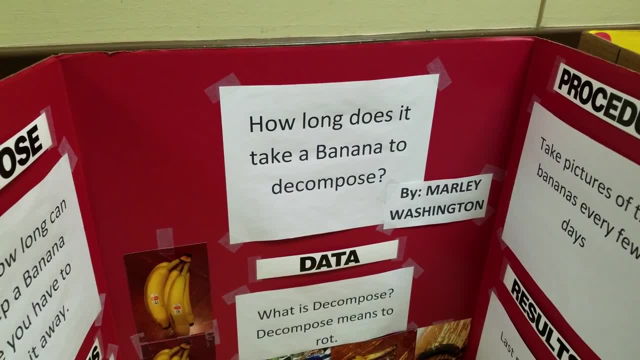 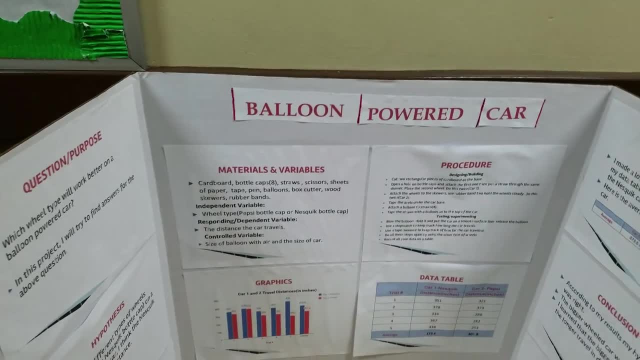 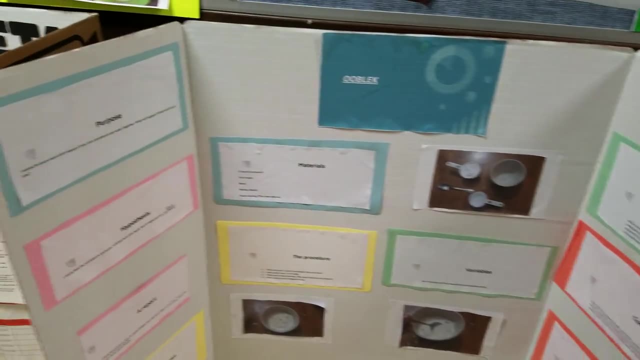 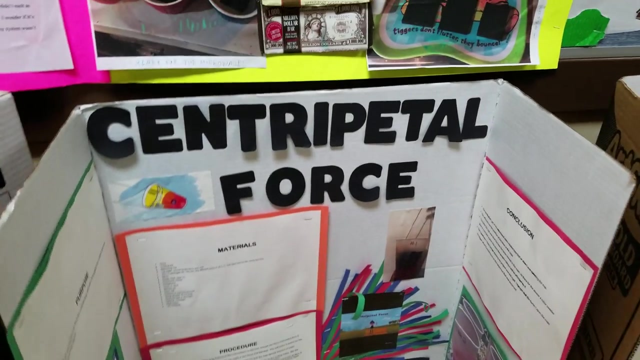 Moving on to how long does it take a banana to decompose? Here is a balloon powered car. Yeah, Oh, looks like a banana. Looks like we have another oblique project. They like it, They like this one. huh, Okay, what is this? 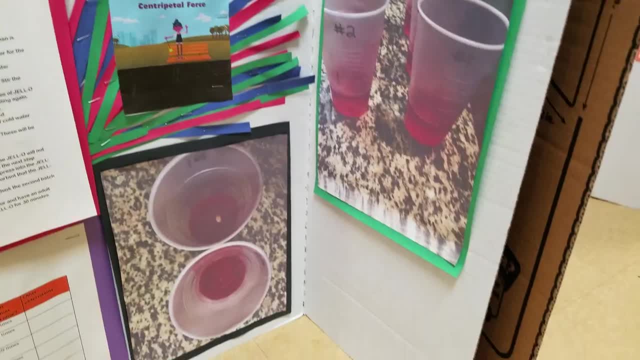 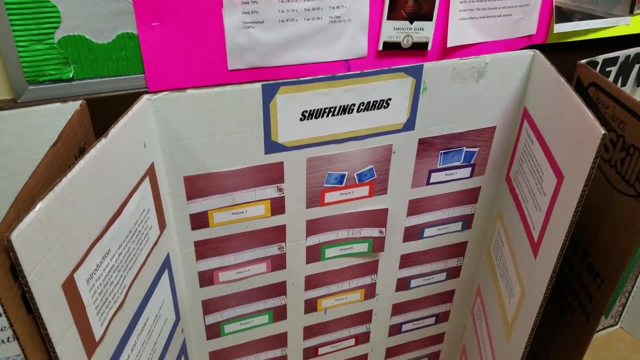 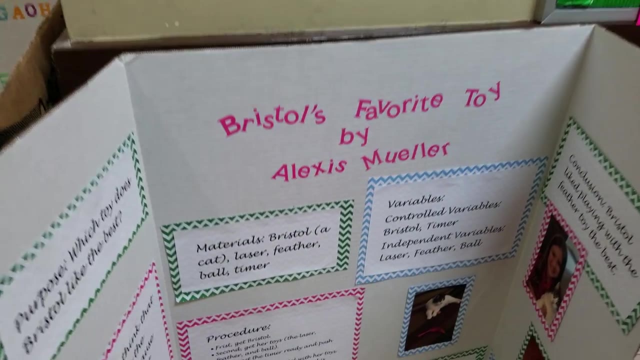 Centripetal force, What's it called Elevator thing? I learned to do this six other times. Here is shuffling cards. Not quite sure of that project, but sure it's interesting. Here we have Bristol's favorite toy. I learned after the first time. 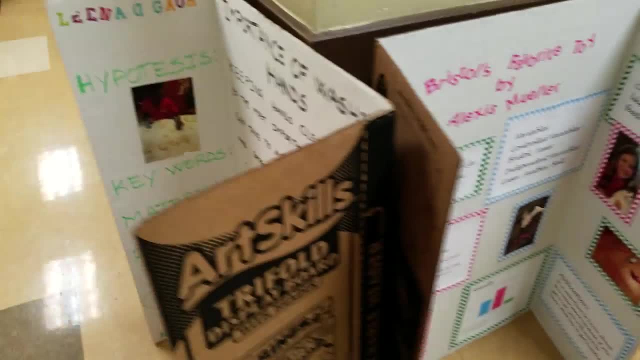 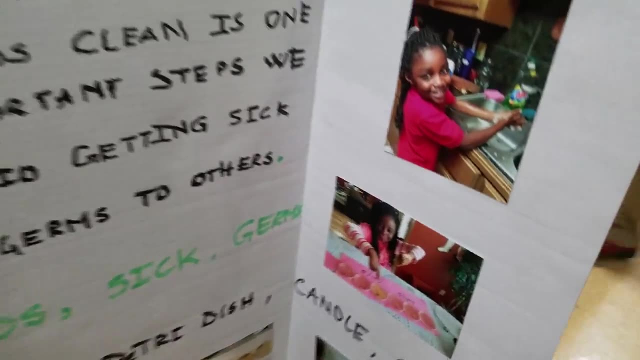 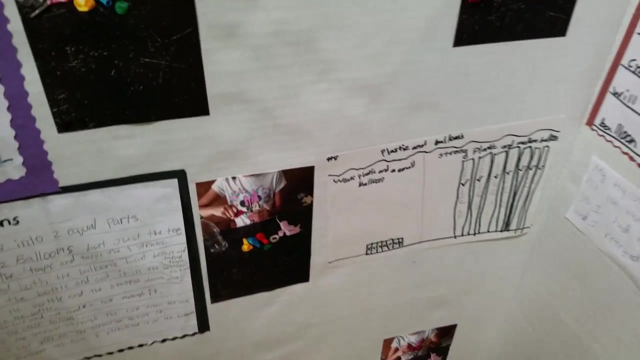 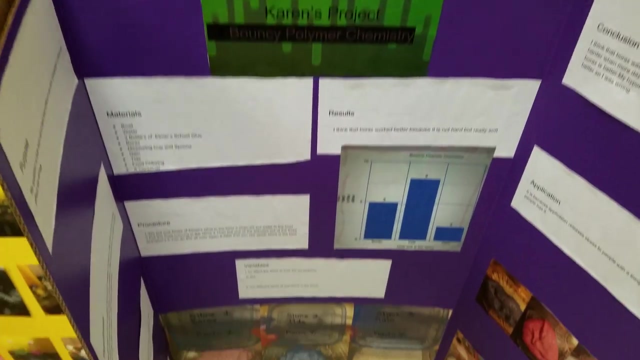 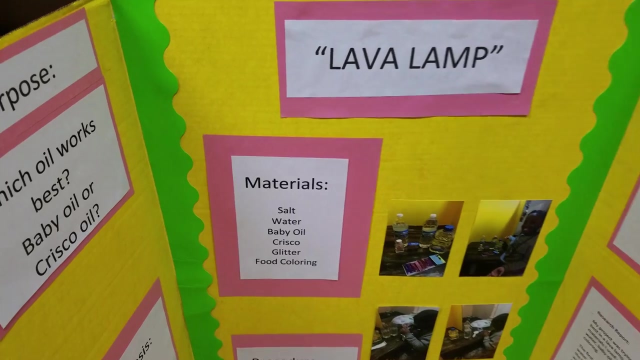 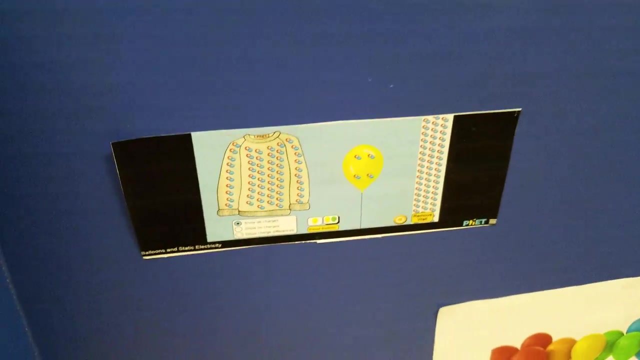 I guess Bristol is the cat. Okay, we have the importance of washing hands. That's a good one. Here we have. how do lungs work? Alright, we have bouncy polymer chemistry. This one is simply titled Lava Lamp Statication, That's the properties of static. 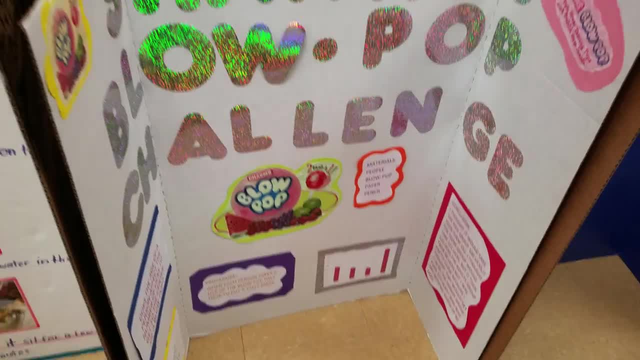 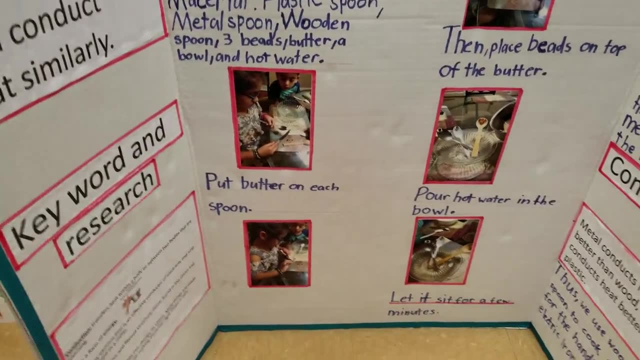 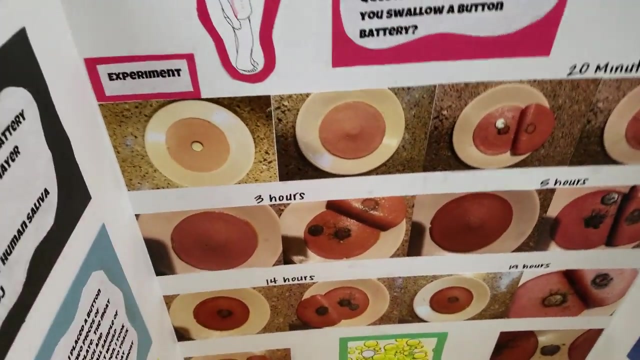 This is a blow pop challenge. Okay, what material conducts heat the most? The air? Okay, here we have belly button battery. Okay, here we have belly button battery. Here we have belly button battery. So You can make up. It was like in the days. 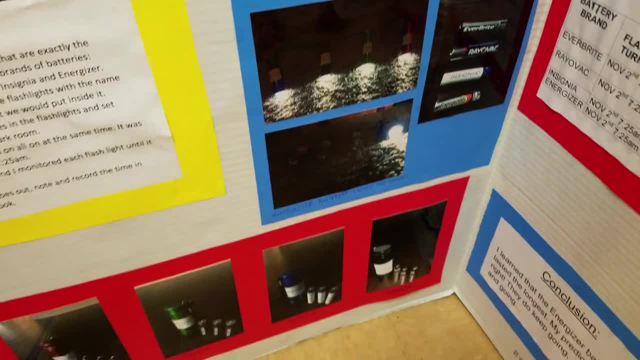 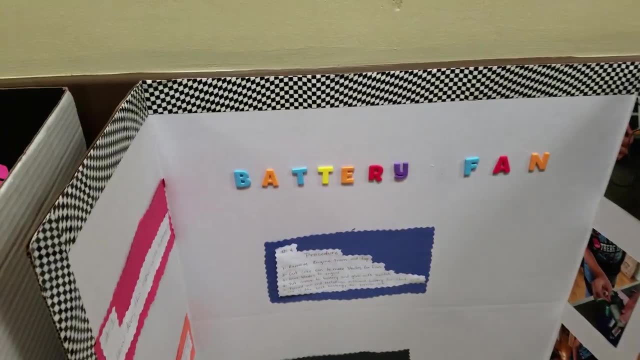 Here we have battery power. You think they created batteries. You think they created batteries, I think. from that one I had to put the glass. Here we have a battery fan, Here we have a battery fan. And then I took, And then I took. 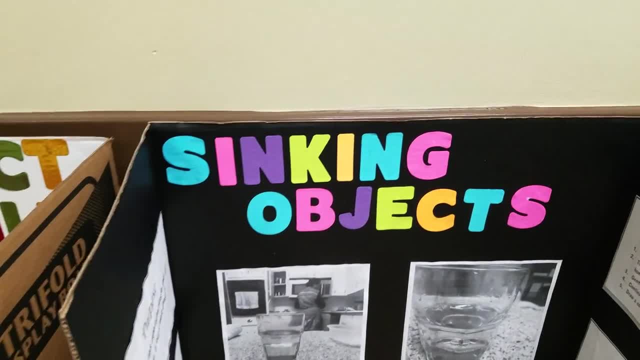 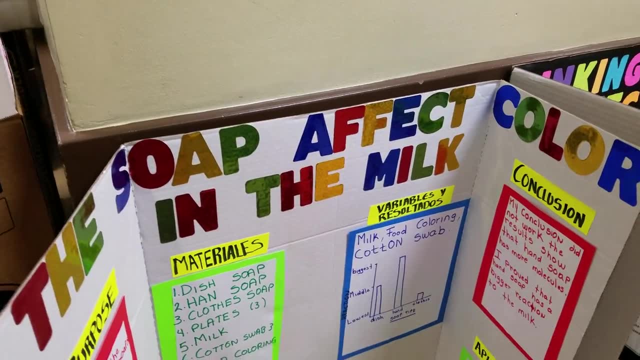 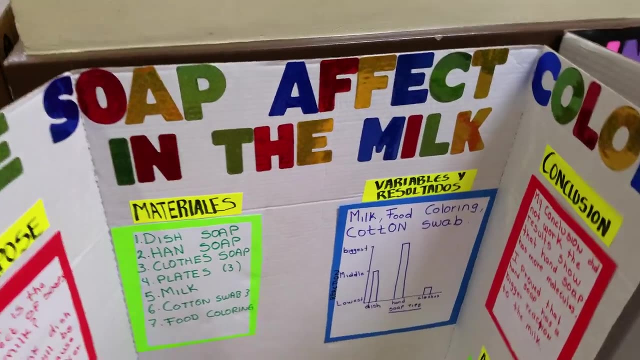 And then I took. This project is titled Sinking Objects. This project is titled The Soap Effect in the Milk. This project is titled The Soap Effect in the Milk. These are K through K through fifth. Yes, Some of these probably from first and second graders. 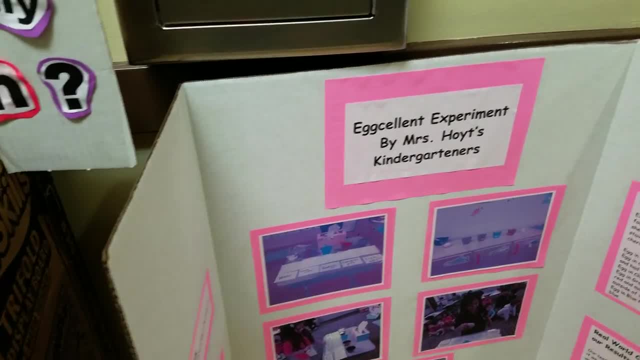 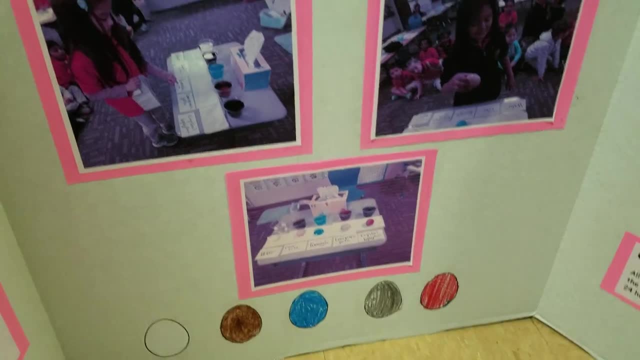 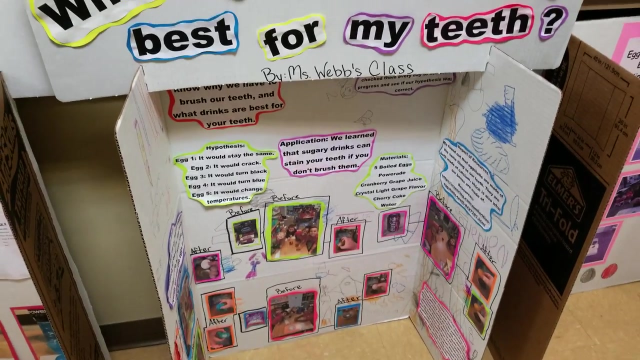 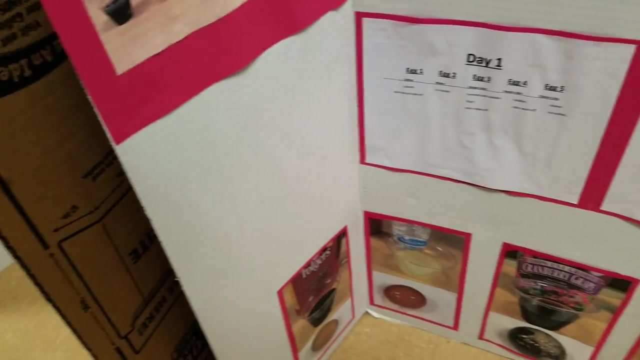 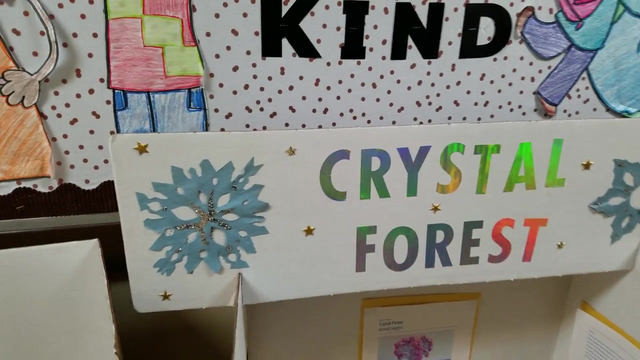 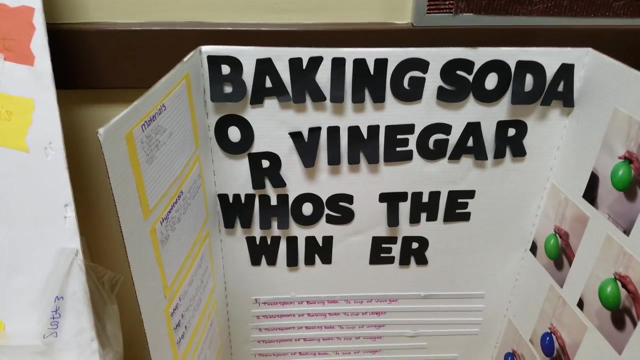 That's why, Okay, this one is titled Excellent Experiment. Okay, this one is titled Excellent Experiment. It's by a kindergartner. Okay, Which drink is exactly best for my teeth? Egg Science Experiment, Crystal Forest, Bacon, Soda or Vinegar? 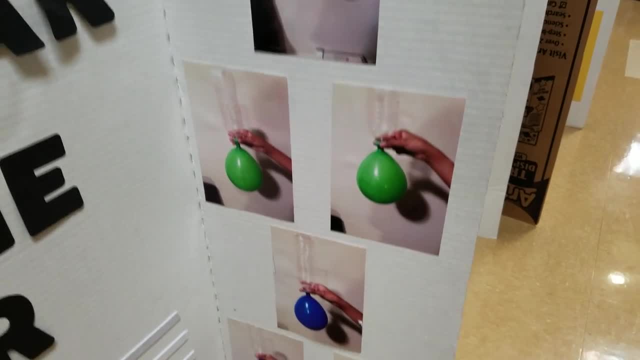 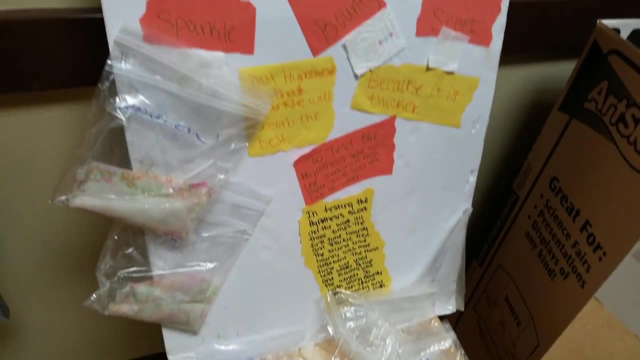 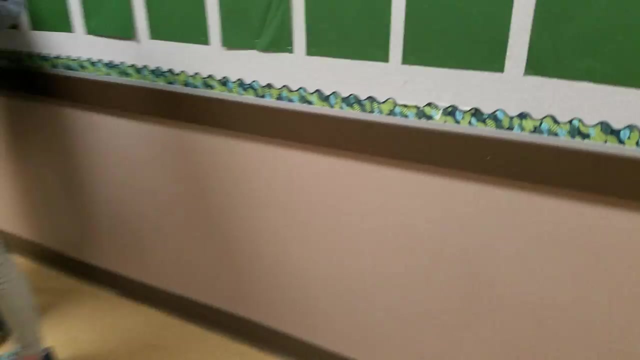 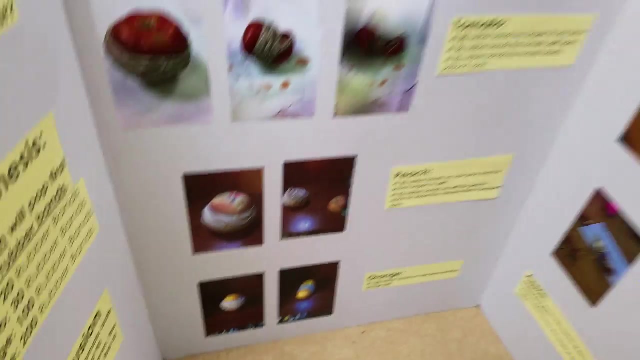 Who wins the who's the winner? I think the end fell off. Who's the winner? Okay, Which paper towel is more absorbent? Got the experiment materials? Okay, This project is titled Popping Fruit. The title of this project is: 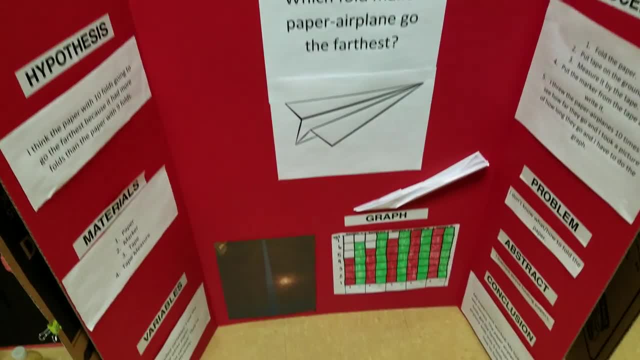 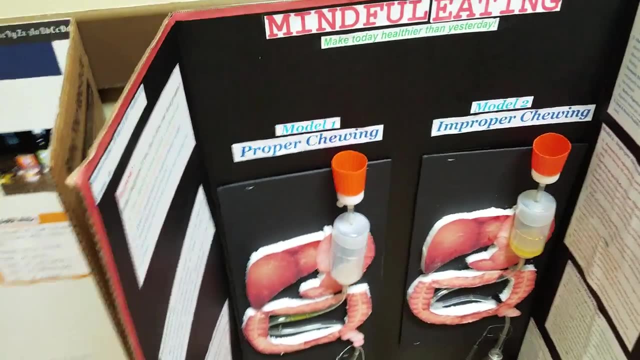 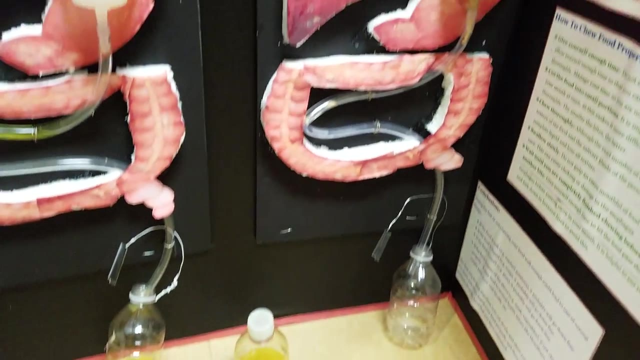 Which Fold Makes Paper Airplane Go the Farthest. Wow, Look at the data. Good, We got a graph down there. Colorful graph. This one is Mindful Eating, Making today healthier than yesterday. Looks like a 3D diagram of a stomach. 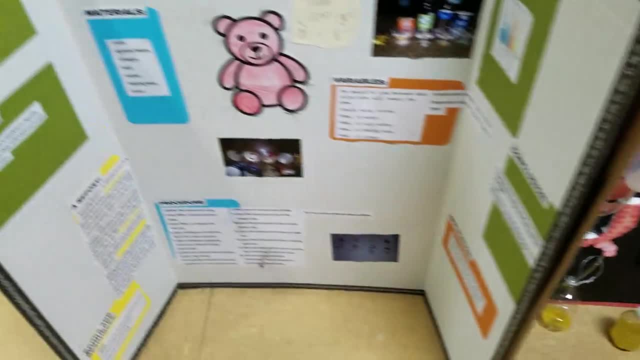 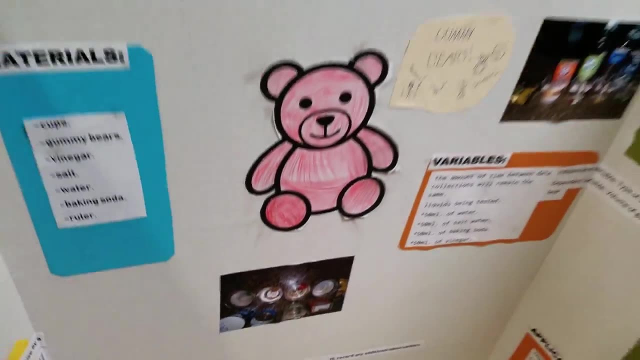 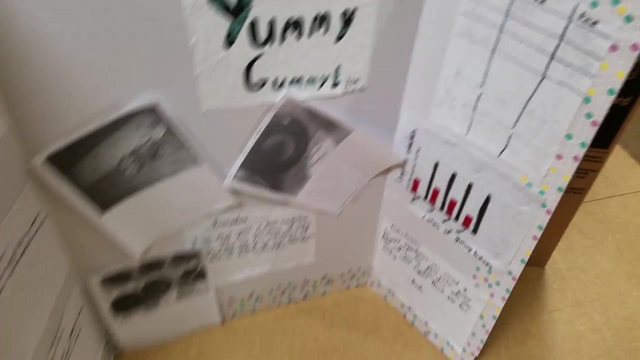 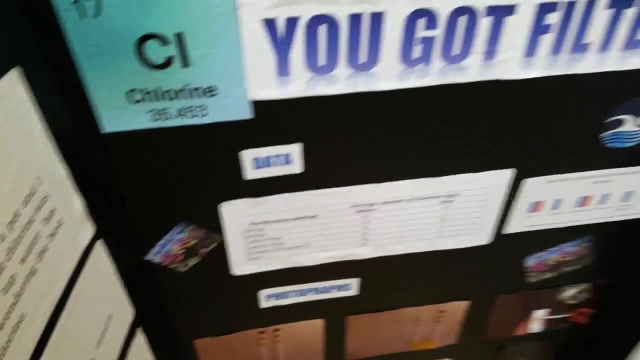 and intestines. This one is called Growing Gummy Bear, Another one, Another one: Yummy Gummy. I thought about you when I saw that. Thanks, That's perfect. Three Here we have You Got Filtered. Look, look, Stop. 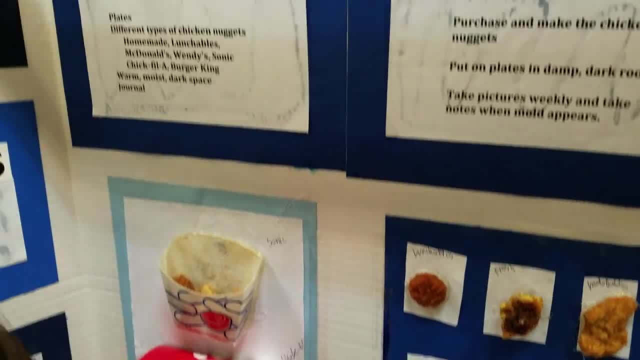 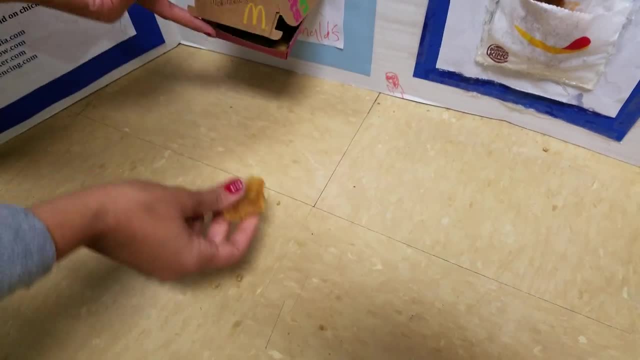 What else do you eat? McDonald's, right? Oh, Look at that. This one is titled Unhappy Meal. Look, Oh, those nuggets. Those nuggets are hard And still greasy, But I still need more That one. 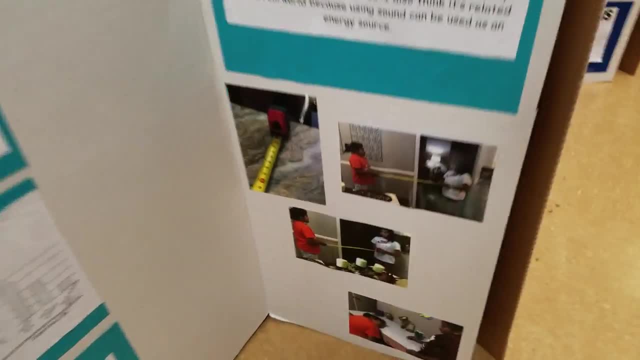 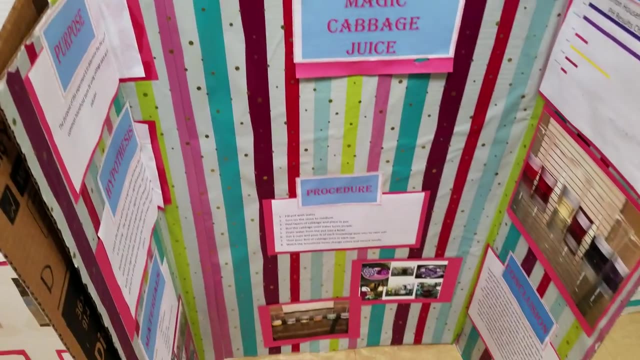 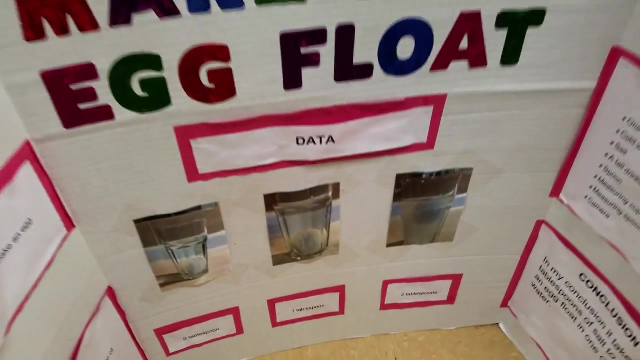 This one is called Medium of Sound Waves. Oh rousy, Oh rousy. Okay, We have magic cabbage juice. It breaks apart. How much salt to make an egg float. Wow, That's what I needed. It's about density, Primitive. 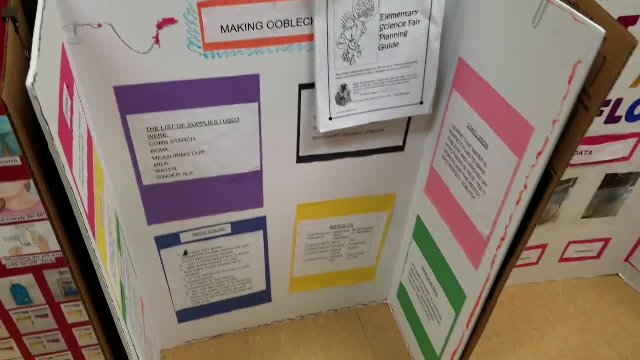 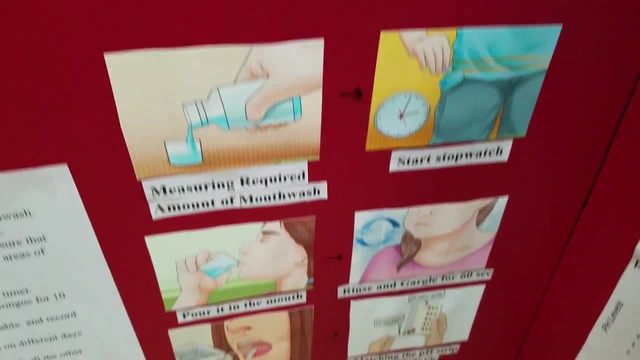 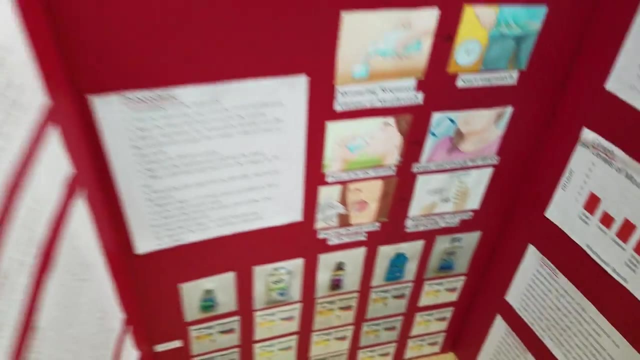 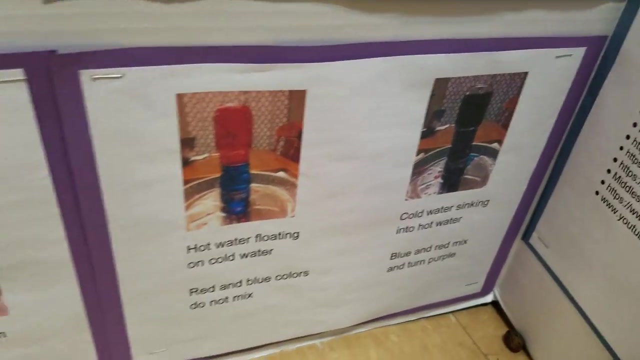 Well, another. We're back to the OWBLEC Making OWBLEC Owbleck. This one is called Mouthwash. Is it safe or not? Here we have water floating on water. It's going to be warm water and cold water because of the density.